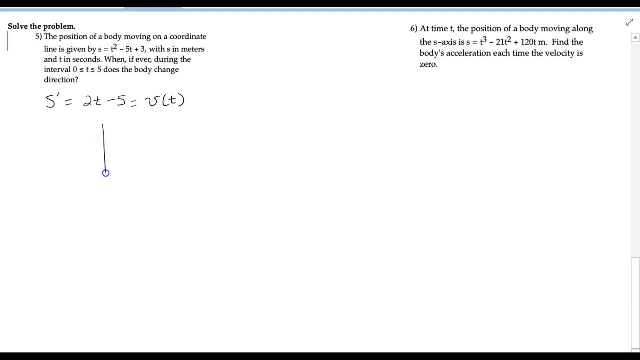 Okay, Now what I'm going to do is I'm actually going to graph that, Because if I graph that, all right, I'll be able to see it very clearly. So let me just make a little grid real quick, Okay. So let's say that it crosses down here at negative 5, right there, Negative 5, point, right there, And then it crosses the axis somewhere right in between here, If you use the rise over the run. 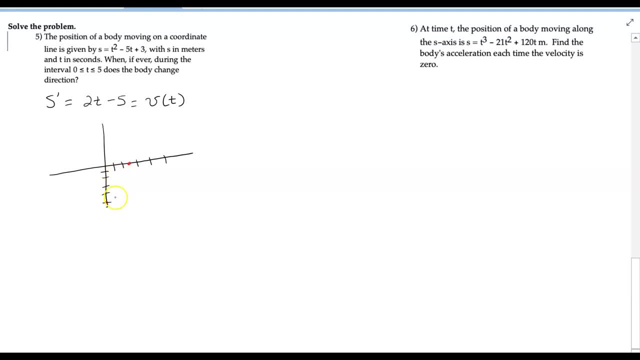 up 2 over 1, up 2.. So up 1, up 2, over 1.. Up 1, up 2, over 1.. You know something like that, So let's just pretend that it crosses right through there. The graph is of course not drawn to scale. All right. 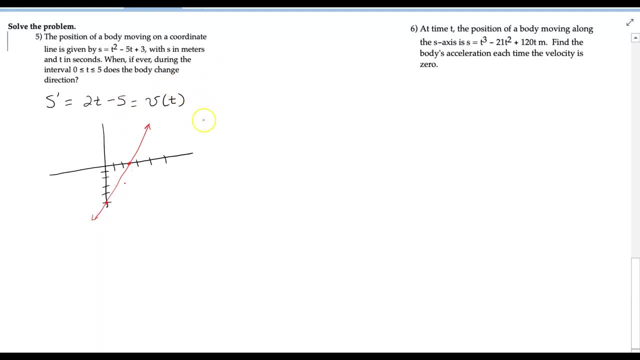 But notice what happens if this is the graph of the velocity. Okay, The velocity is positive above the axis And it is negative below the axis. So this is the graph of the velocity versus time. So where does it change direction? Right there, at that point. And in order to figure that out, all you have to do 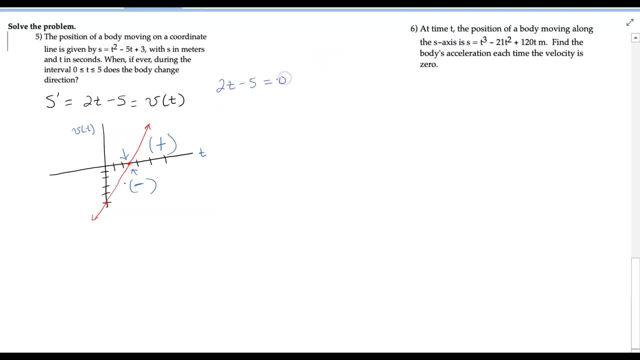 is: take your 2t minus 5 and you set it equal to 0. So we get 2t equals 5 and we divide both sides by 2.. It happens at 5 over 2 seconds, which is 2.5.. So we can say that it changes direction. 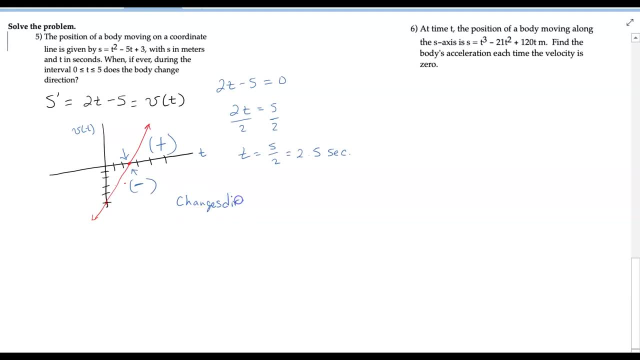 changes direction at t equals 2.5 seconds. All right, so that's where it happens. All right, that's that. That's the first problem for particle motion. Now let's take a look at another problem. Just draw a little dividing line here, All right. in the second example. 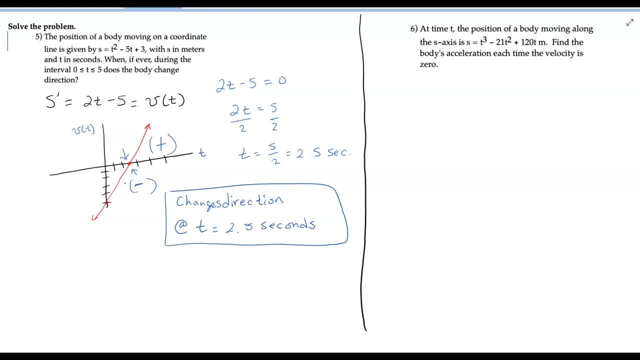 they say, at the time t, the position of a body is moving along the s-axis. where s is equal to t cubed minus 21t squared plus 120t meters, It says: find the body's acceleration each time the velocity is 0.. So what are we going to have to do? First, we have to find s prime of t. 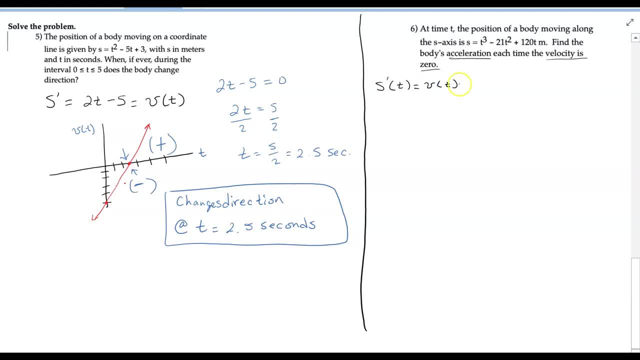 which is the velocity. And once we find the velocity function, we're going to set it equal to 0 and figure out those two time values, or three time values- There's two actually- Then we're going to plug that into the second derivative of the position function, which is the acceleration function. So it's kind 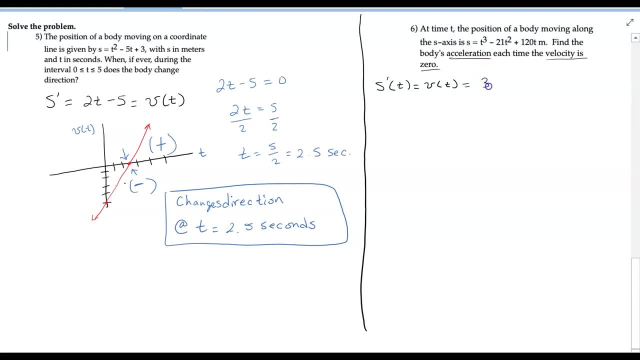 of a combination problem here. First derivative: the velocity is 3t squared minus 42t plus 120.. Okay, so this one. right here we're going to have to set it equal to 0, because this is where the velocity equals 0.. So I'm going to factor out the 3, because 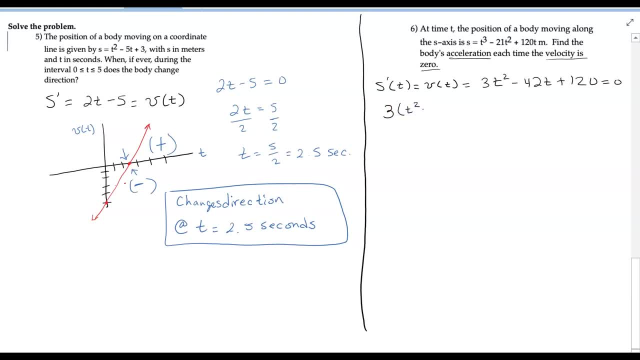 it's the greatest common factor. It's going to leave me with t squared minus 14t plus 40.. All right, and now this right here, I'm going to go ahead and I'm going to factor set it equal to 0. 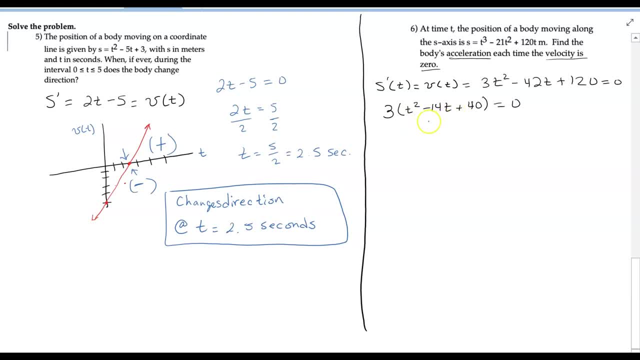 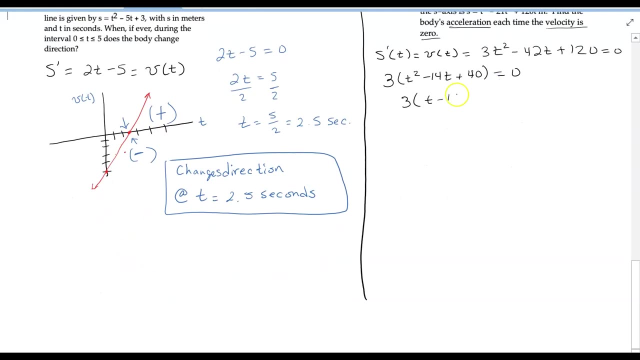 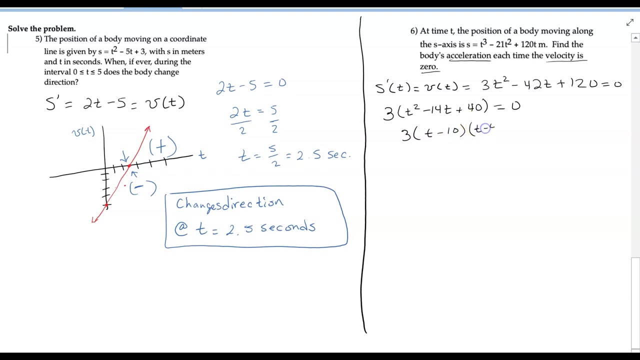 and I'm going to factor it out: Factors of 40 that add to give me negative 14,. well, that's not too difficult, That is 10.. Oops, Second there, messing with my pen here, That is negative 10 and negative 4.. So it looks. 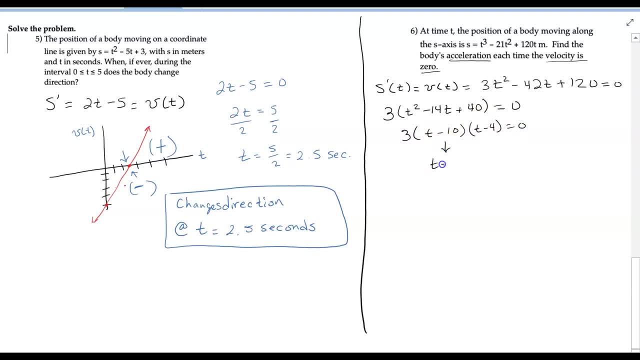 something like that. All right, So I get a time t equals 10 and a time t equals 4.. This is where my velocity is 0. But now they want us to find the acceleration when the velocity is 0. So what we're going to? 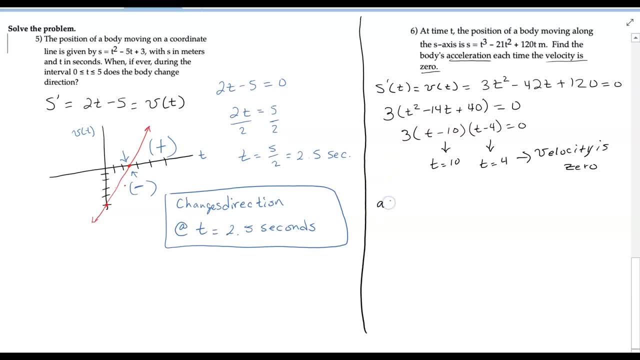 have to do is we're going to have to take the derivative one more time. We have a of t, which is s double prime of t, which is v prime of t, which is the first derivative of the velocity function, or the second derivative of the position function, And so we're going to get 6t minus 42.. 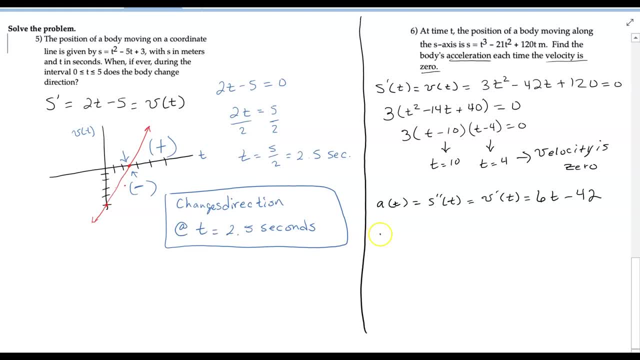 6t minus 42.. And so to find the acceleration, we're going to plug in 4 into 6t minus 42, the acceleration function Six times four minus 42 equals 24 minus 42, which is negative 18 meters per second squared. So that's the first one, That's the first.